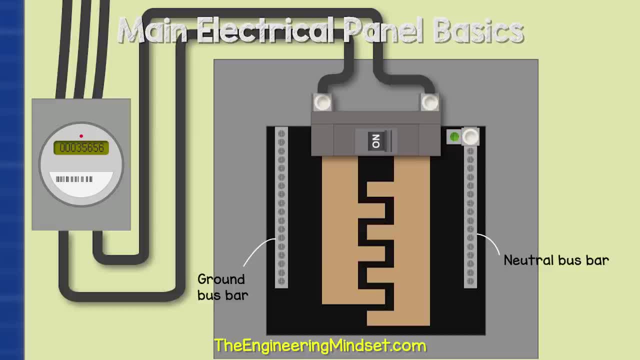 holes and the screws will lock them in place. In this example, we have a block on either side of the panel. As this is a main panel, the two busbars can be joined together, So we have a connector bar between them. That. 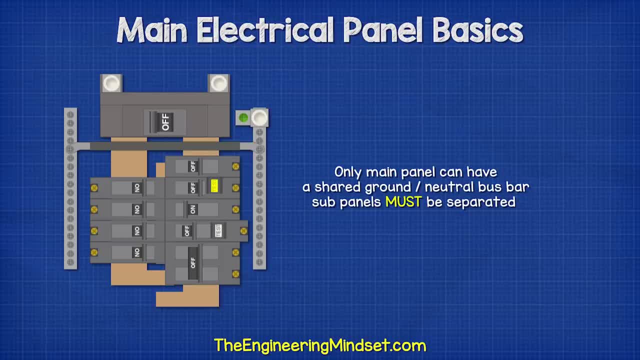 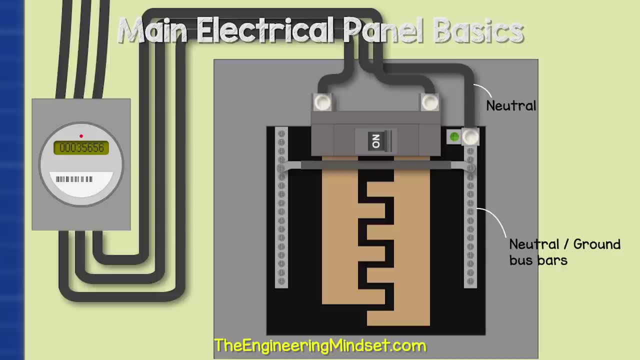 way we have a shared neutral ground busbar. The vast majority of the signals should be dependent properly. Subpanels must have their bars separated, but that's a topic for a separate video From the electricity meter. we will have the neutral wire connected to the lug on the top. 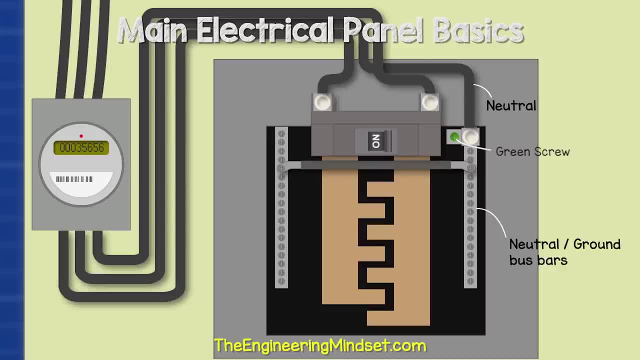 of the neutral ground bar. Notice the green screw. This is bonding the neutral bar to the metal casing of the service panel. The purpose of the neutral bar is to return the electricity to the transformer. It actually does get a bit more advanced than that, but we're going to look at that in a 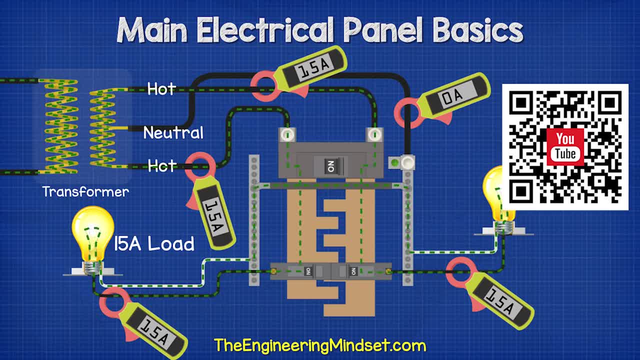 more advanced video. This is just covering some of the basics here, But it may not be exactly that new, but maybe another thing worth considering. when it's available, Two hot wires will provide the electricity and once it is used it will return to the. 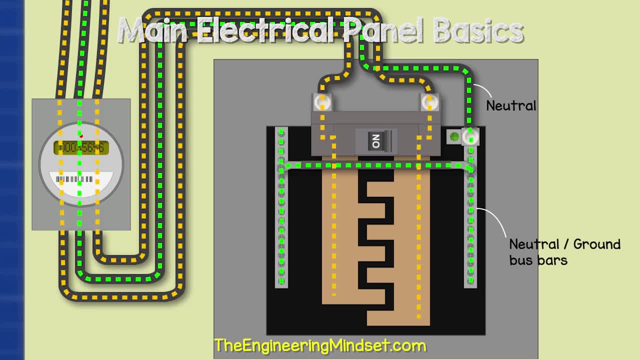 transformer via the neutral bar. It is still AC alternating current, but to make it easier to visualise, I've only animated the current flowing in one direction so you can see the path it will take. Now if we were to take our multimeter and connect one lead to the bus bar and the other. 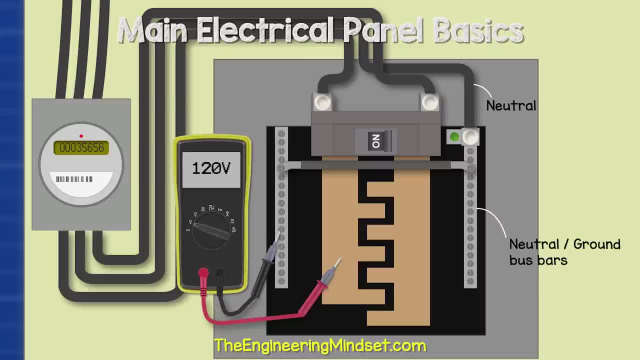 lead to the neutral bar, we would get a reading of around 120 volts. If we connect the multimeter leads to the other bus bar and the neutral bar, we would again get a reading of around 120 volts. But if we connect the multimeter leads to the two bus bars, then we get a reading of: 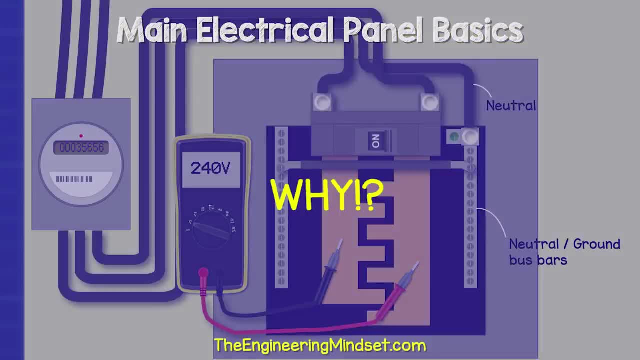 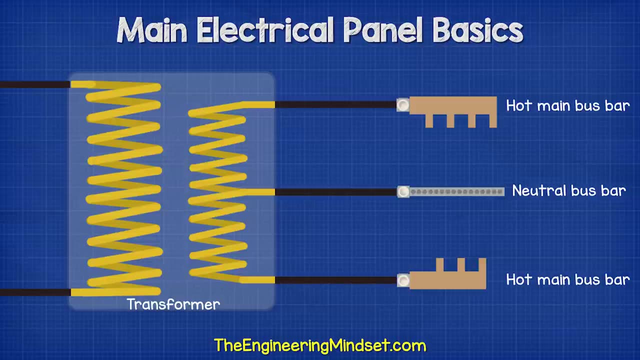 double that at around 240 volts. So why is that What's happening here? So when we look at how the transformer is connected to the main panel, we have the two hot bus bars connected to either end of the secondary coil in the transformer. 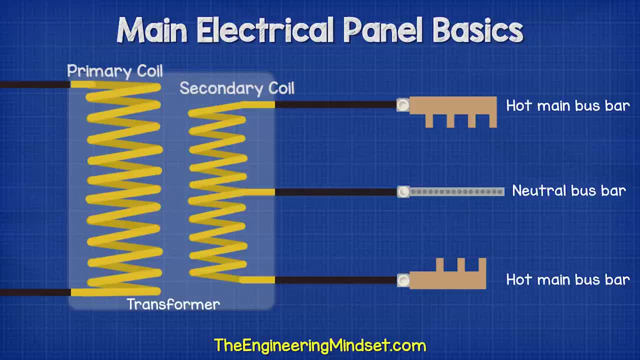 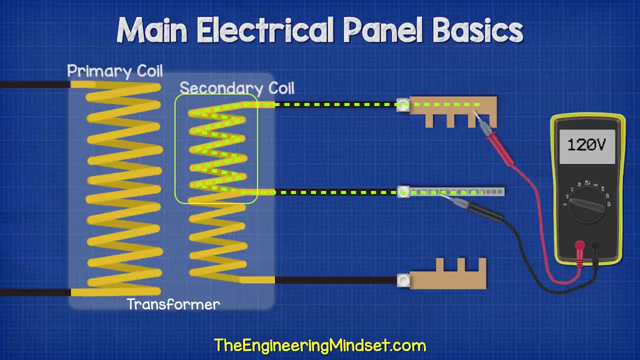 And then we take the neutral bus bar connected to the centre of the secondary coil. So basically, when we connect across the bus bar and the neutral bar, we're actually only using half of the coil, so we are only picking up half the electrical voltage the transformer can provide. so that way we get 120 volts. 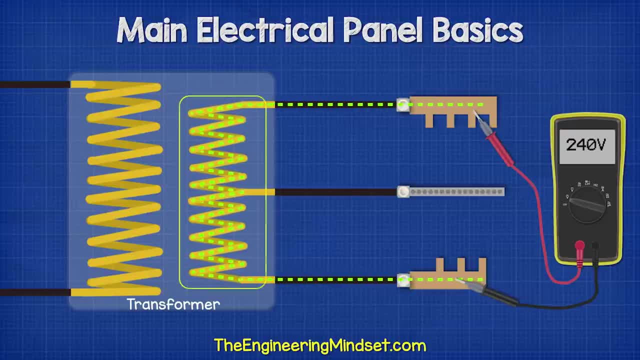 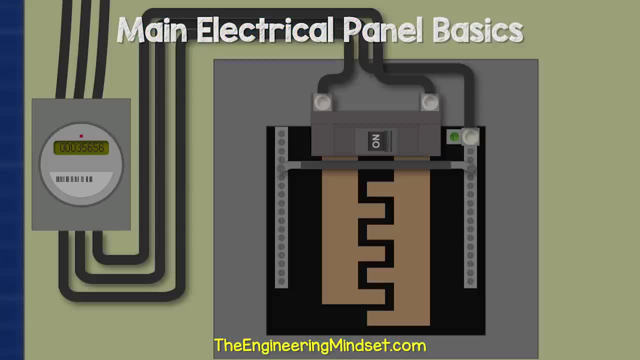 When we connect to the two bus bars, we're connecting to the full length of the coil, so we're picking up the full voltage which the transformer can provide. Therefore we get 240 volts. Now coming back to the panel connected to the bus bar, we'll have our circuit breakers. 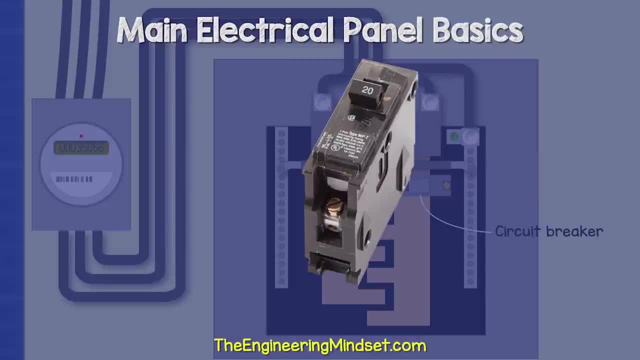 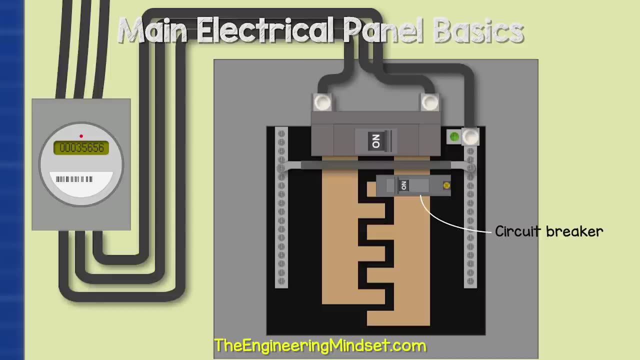 These will look something like this, with this black plastic casing and a toggle switch on top. The circuit breaker controls the flow of electricity into individual circuits in the property. It can be manually tripped to cut the power. but it also has two important features. 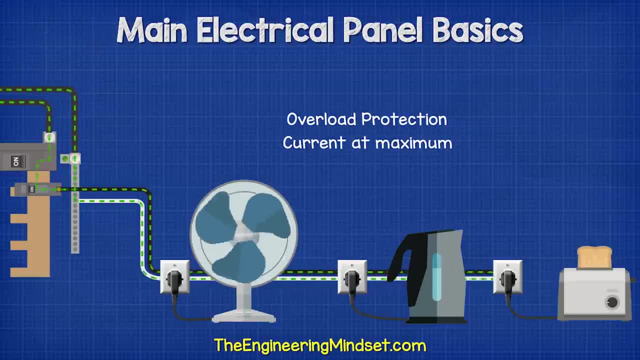 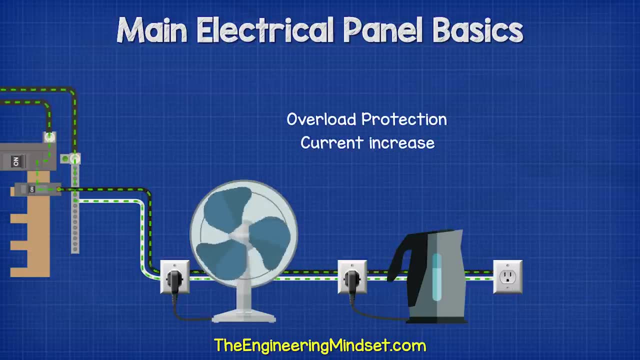 The first feature is overload protection. The circuit breaker is rated to handle a set amount of electrical current. When appliances or lights are connected to the circuit, they will each increase the current in the circuit. If too many things are plugged in and turned on, then eventually the current will be more. 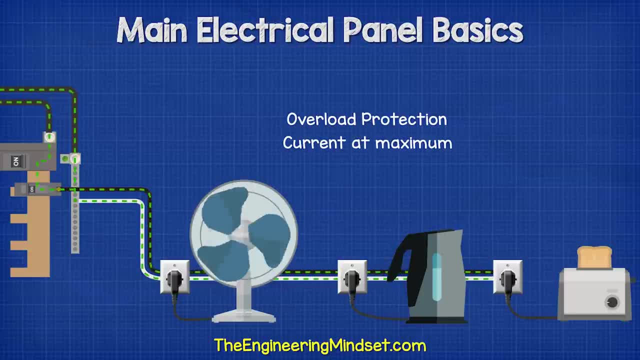 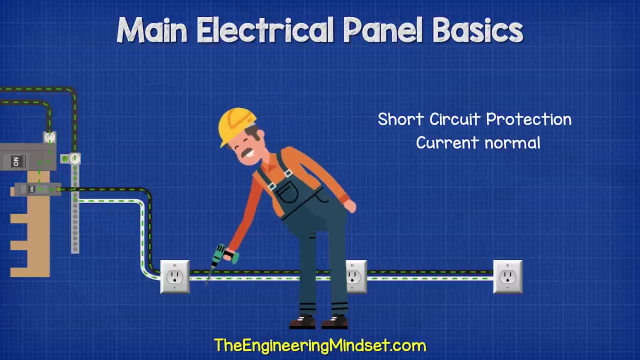 than the breaker can handle and the breaker will automatically trip to cut the power and power off to the circuit and protect the property. The second feature is short circuit protection. When the hot and neutral come into direct contact with each other, the current will dramatically increase almost instantly. 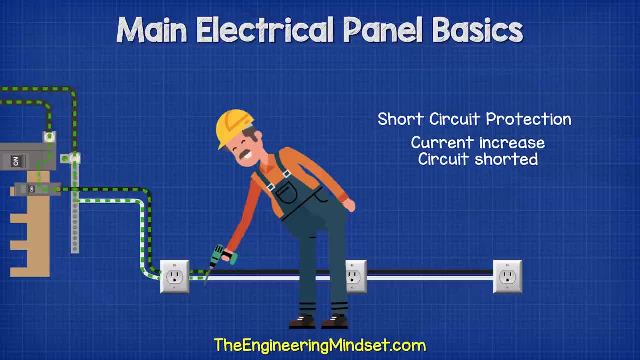 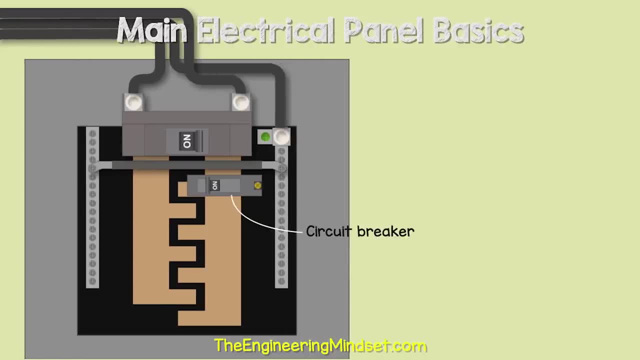 When this occurs, it creates a magnetic field which will trip the breaker and cut the power automatically. Let's have a look at how the circuit breaker is connected to the electrical circuit. In this example, we will connect to a simple light fitting which is controlled by a switch. 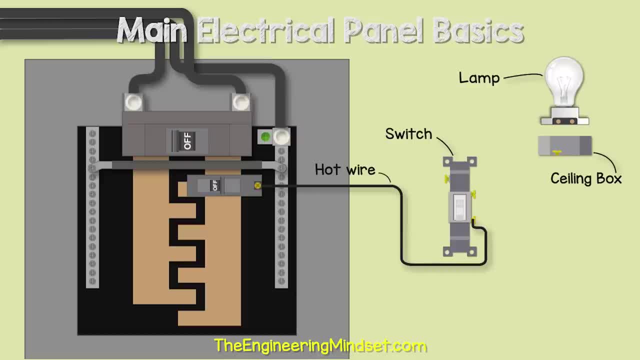 We take the hot wire from the circuit breaker and run this to the circuit breaker. The circuit breaker is connected to the electrical circuit. We connect this to the switch. We then run another wire from the switch and over to the light fitting. From the light fitting we have a neutral wire which carries the return current back to the 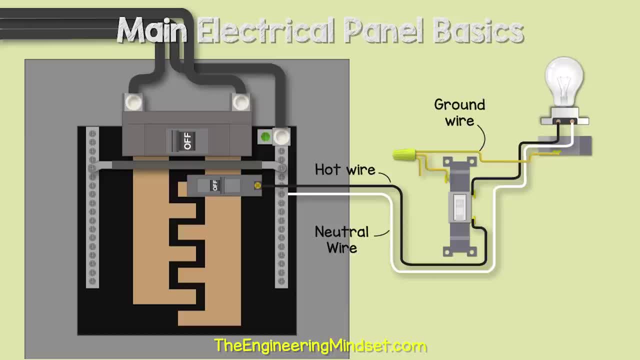 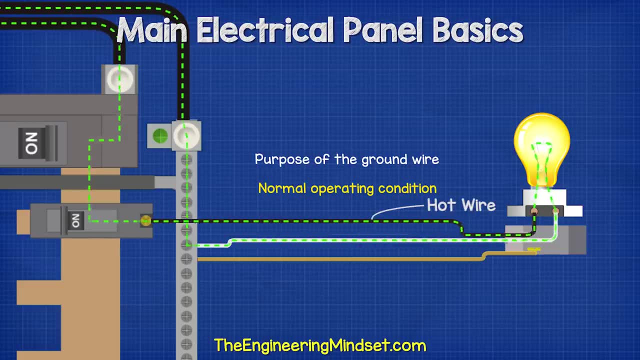 neutral bus bar. We take the ground wire from the metal casing of the ceiling box and the switch and we also join this to the neutral bus bar, as in this case it's shared. The purpose of the hot wire is to carry the electrical current over to the light fitting. 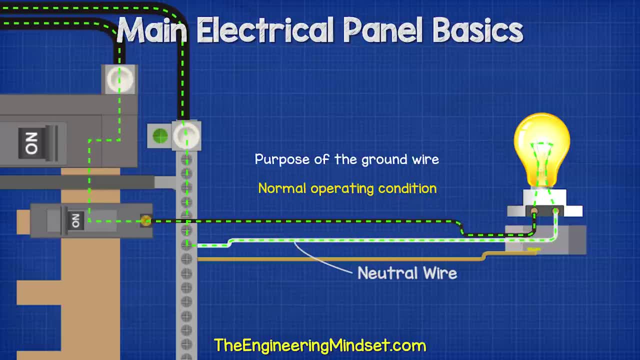 The purpose of the neutral wire is to carry the used electrical current back to the main panel and then back to the transformer. The purpose of the ground wire is to provide protection for a fault current If, for example, the hot wire came loose and touched the metal casing of the light fitting. 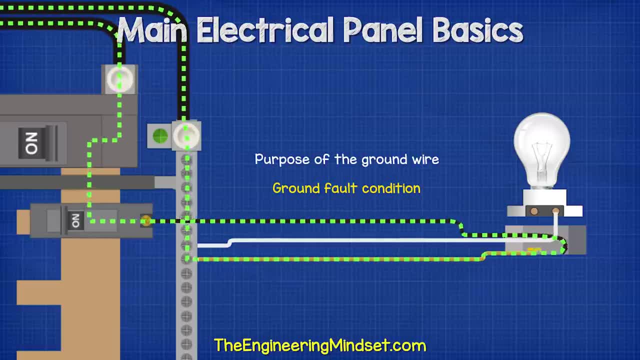 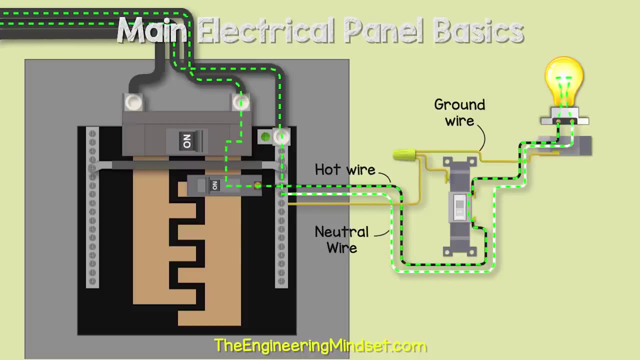 the ground wire provides a low resistance path back to the panel. Without this path, electricity could flow through you. if you touch the metal box, As the current flows through the ground wire, it will increase the current and that will trip the breaker automatically. So the electricity flows through the hot wire, through the main breaker, down the main bus. 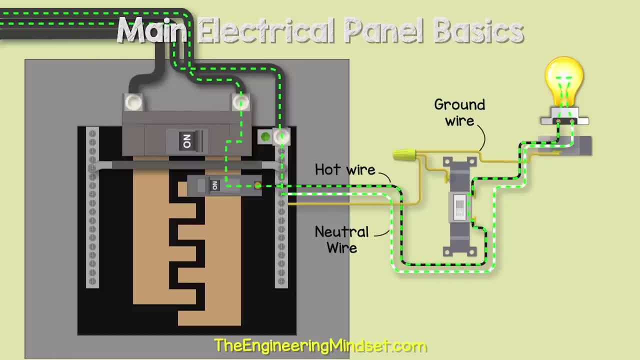 bar and into the circuit breaker. From there it flows along the hot wire, across the switch and light, then back along the neutral wire and into the neutral bus bar, along the neutral bus bar wire and back to the transformer. I've animated this using AC alternating current but to make it easier to understand the path. 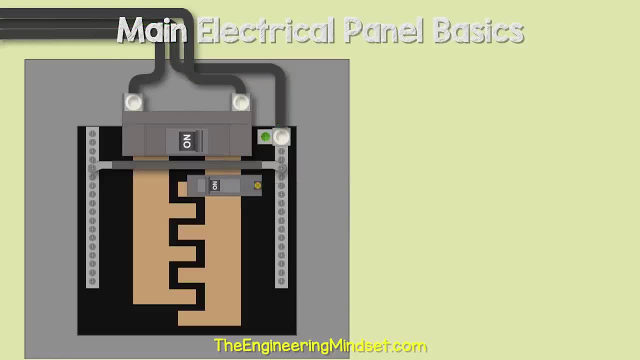 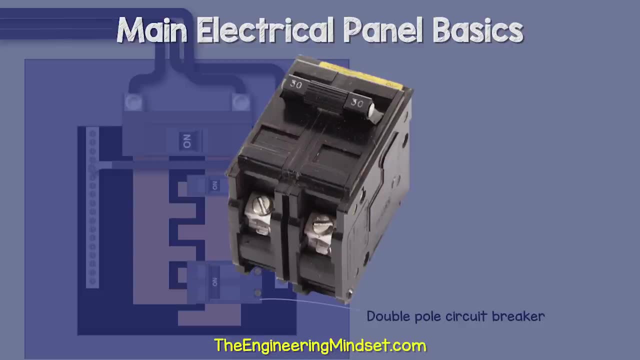 I've shown it flowing in a single direction now. Ok, so what else might we find here? We might find a double pole circuit breaker which will let us connect to both bus bars to get 240 volts which we can use to power larger appliances like dryers, routers and 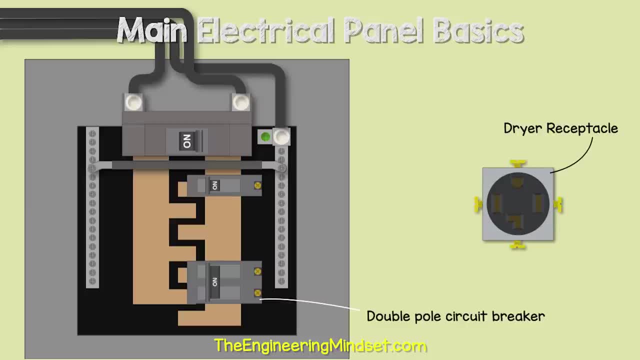 wires, ranges and air conditioning units. If we look at the dryer circuit example, we run the red hot wire from the circuit breaker which is connected to the main bus bar number 2, and we run this to the receptacle. Then we run our black hot wire from the other terminal of the circuit breaker, which is connected 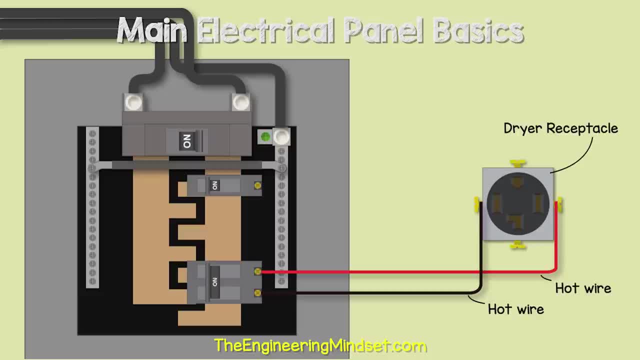 to bus bar 1 and we connect that to the receptacle. also, In this case we have the neutral wire connected between the neutral bus bar and the receptacle, which will allow us to get either 120 or 240 volts from the outlet. Then we have a ground wire to provide a safe route for any fault current. 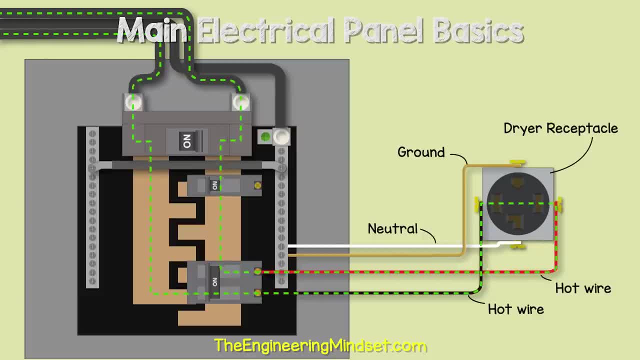 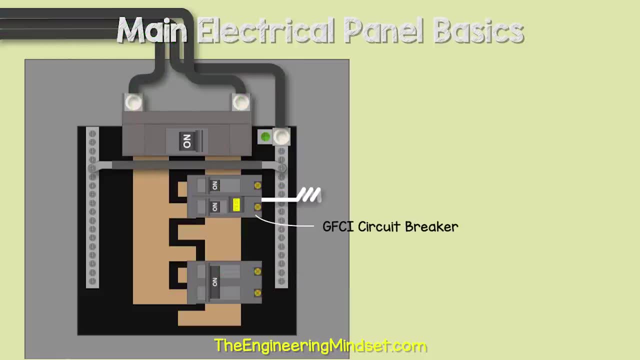 Now we can either connect across the two hot wires for our 240 volt connection or between the hot wire and the neutral wire to get 120 volt connection. We will also very likely find a GFCI circuit breaker, which stands for ground fault circuit. 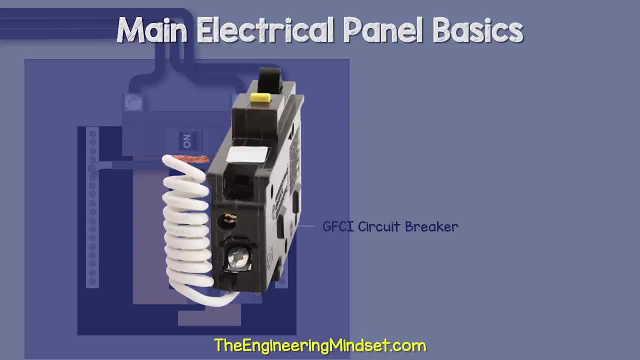 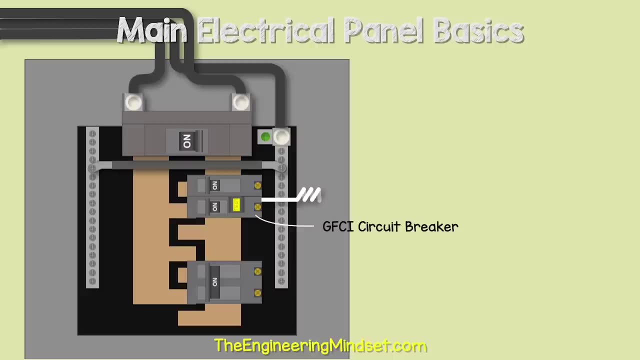 interrupter. This will look something like this and, depending on the model you buy, you will usually have a pigtail neutral wire connected to it. GFCIs are required on certain circuits where outlets are used for places like kitchens, bathrooms, hot tubs, etc. 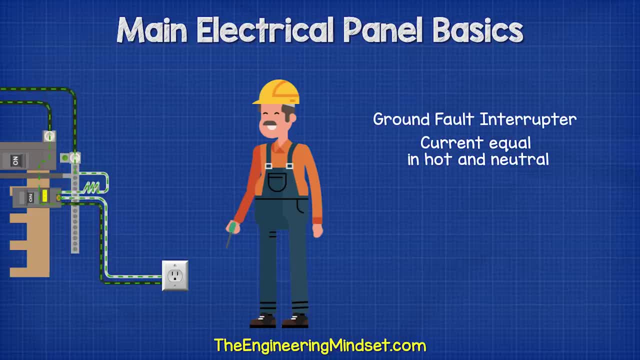 You should check with the national electric code for exact details. The GFCI breaker has both the hot and the neutral flowing through it. This way you can measure the current flowing through both wires and ensure they are equal. If we took a standard outlet, we would take our hot wire from the breaker and connect. 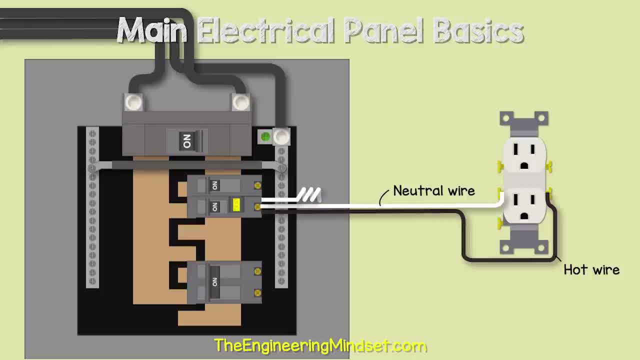 this to the outlet terminal. Then we take the neutral wire and run this back directly to the circuit breaker to a specific neutral terminal. We then connect the pigtail wire into the neutral bus bar. This will provide the return path And of course, we run the ground wire from the outlet back to the neutral ground bar. 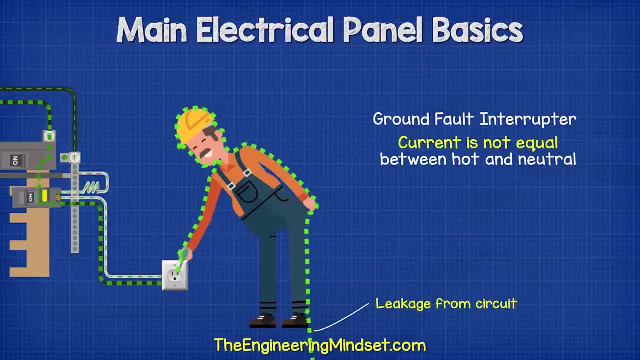 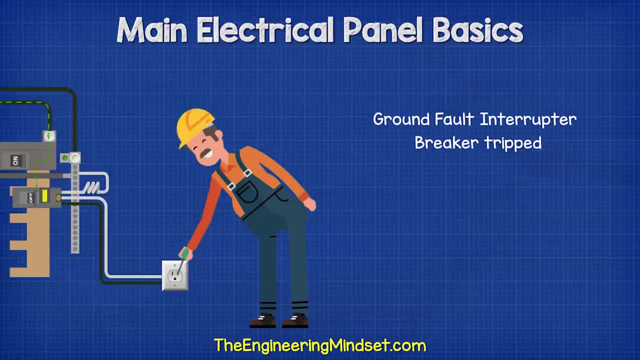 If we look at this example, the current is flowing normally until the guy sticks a screwdriver into the socket. The electricity then flows through him instead of the neutral wire. The GFCI is measuring the current in the two wires and notices that these are not equal. 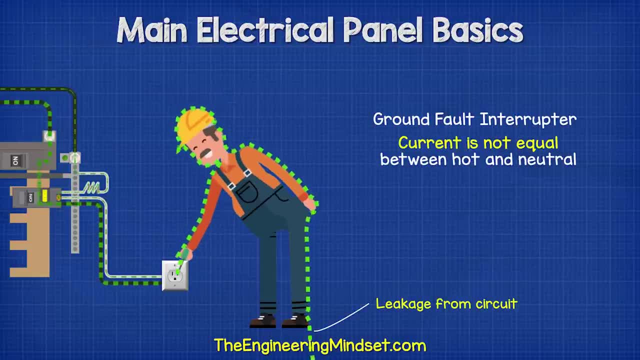 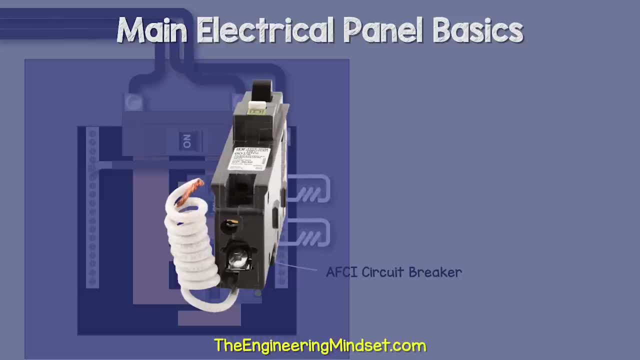 It then automatically trips the breaker to cut the power and save the man's life. We might also come across an AFCI circuit breaker. This stands for Arc Fault Circuit Interrupter. These are required for circuits feeding bedrooms, hallways, kitchens, etc. 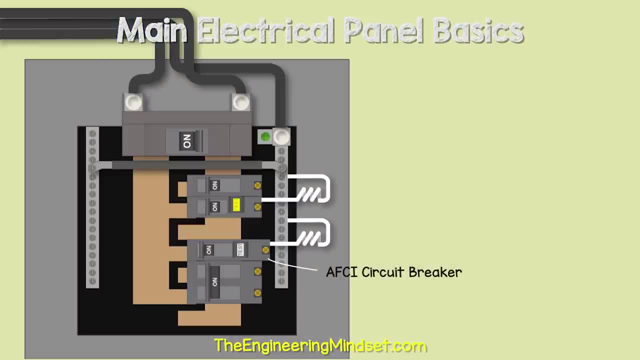 Again, check with the National Electric Code for exact details. AFCIs work also by being connected to both the hot and neutral wires. Inside this circuit breaker is a circuit board which is measuring the circuit and monitoring for patterns which indicate an arc fault is occurring. 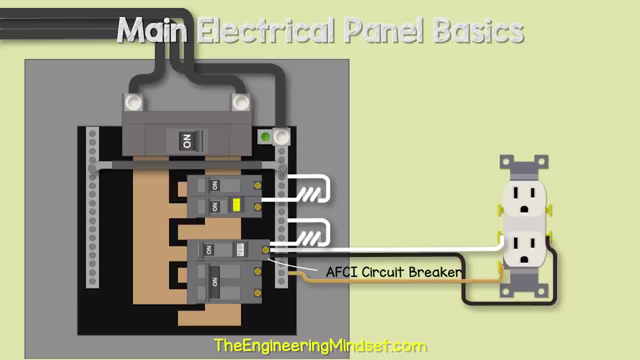 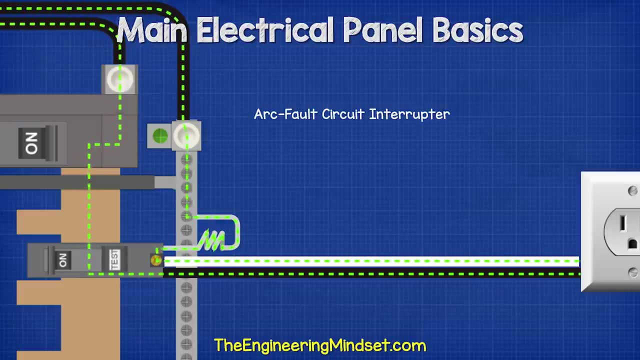 These are installed pretty much identically to how we saw the GFCI breaker. Under normal conditions The current flows through the hot, back through the neutral into the breaker, then through the pigtail and back through the neutral bar. But if, for example, a screw was accidentally inserted very close to the cable and removed, 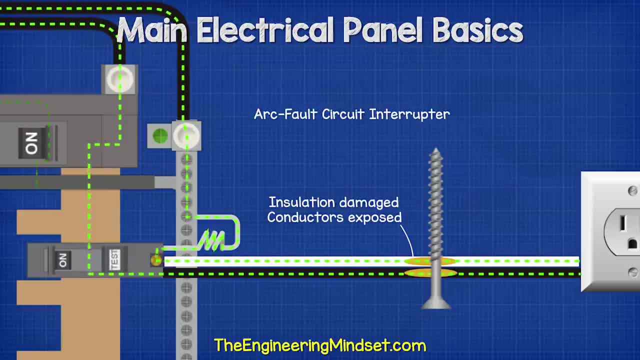 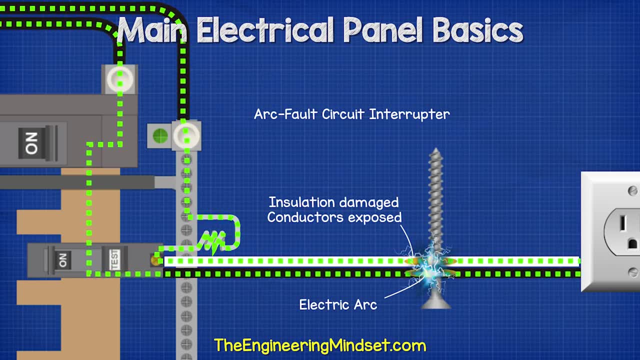 the insulation to expose the copper wires. the electricity could now potentially jump across or arc from the hot wire and into the neutral. The arc is incredibly hot and causes most residential electrical fires. As the arc occurs, it creates a unique signal in the electrical cable. 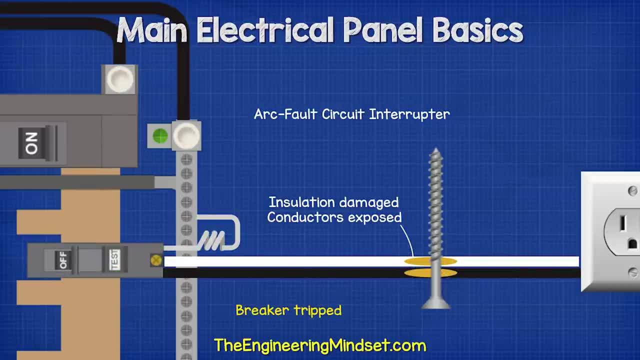 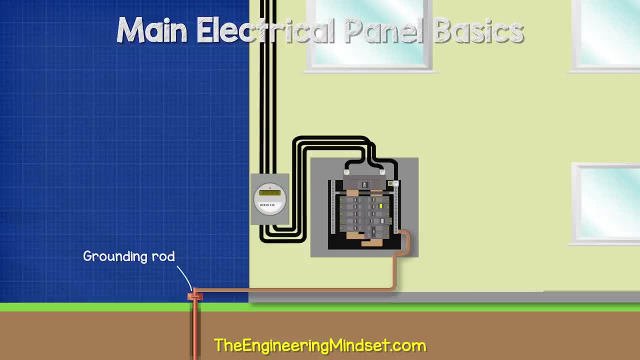 The circuit breaker can detect this signal, It will automatically trip to cut the power. Connected to the neutral ground bar will be a thick, uninsulated copper wire which runs out of the bottom of the panel and off to the ground rod which is pushed into the earth. 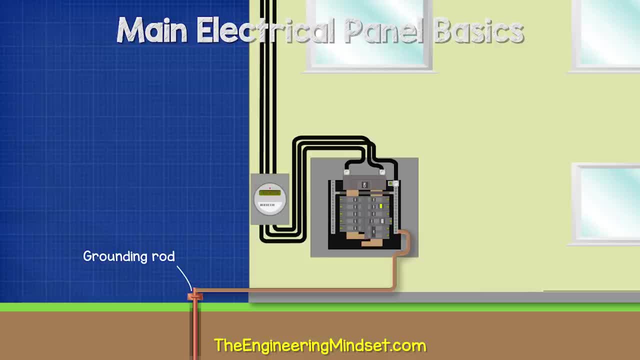 near the property. Under normal circumstances, no electrical current will flow through this wire. Its purpose is to dissipate high static voltages from things like lightning. This way, the electrical systems and equipment is protected from damage. Additionally, we will also find a bonding wire to metal pipework in the bottom of the